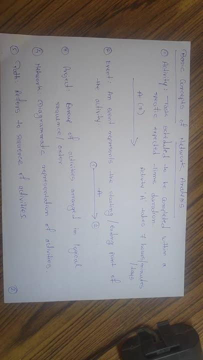 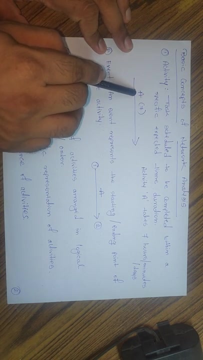 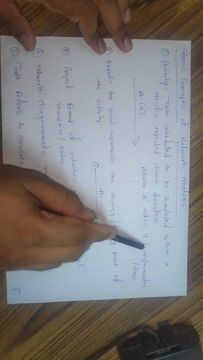 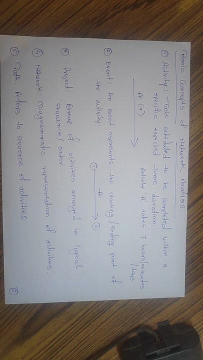 the time duration, which is called activity, And it is represented like this With the help of arrow. A, is activity and it takes 7 units. Now this unit may be specified in the problem. It could be 7 hours, 7 minutes, 7 days. Whatever may be the unit of the given. 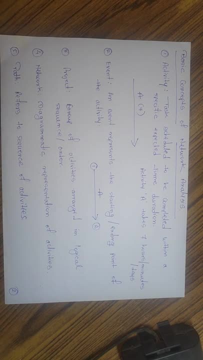 quantity that will be specified in the problem. So the unit of the given quantity that will be specified in the problem. So the unit of the given quantity that will be specified in the problem, This 7 means just a unit. It will be specified in the problem. So activity. 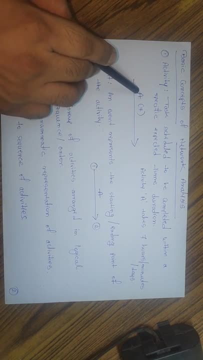 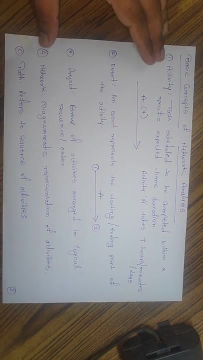 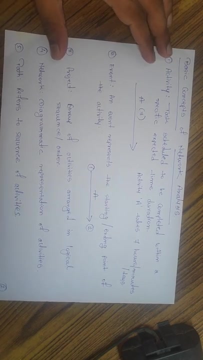 will represent like this. It means now A activity will take 7 units of time. Next concept is event, And event represents the starting, ending point of the activity. Now, this activity starts from this point and ends at this point. So this activity starts from this point and. 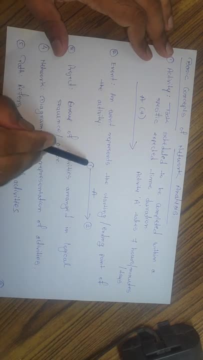 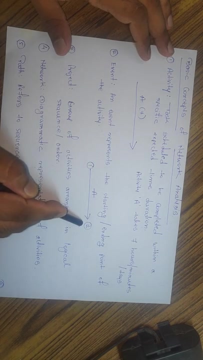 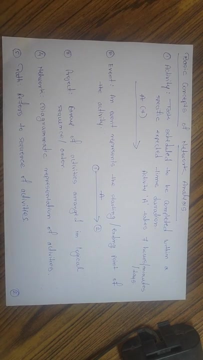 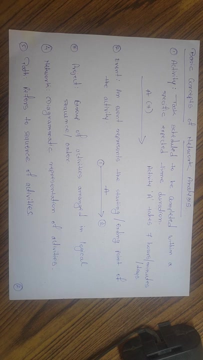 ends at this point. So event is this, one is event and two is also one event. A, this one is starting event and two we can call an ending event, And activity is represented by these two nodes. Third basic concept is project, Group of activities. 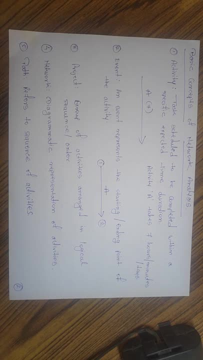 arranged in logical sequence or order is called project. Now, what could be the project? For example, we want to transport something from Mumbai to Delhi, Then the project might list down the activities like transportation, loading, unloading, maintenance and so on. All these activities are represented in a sequential 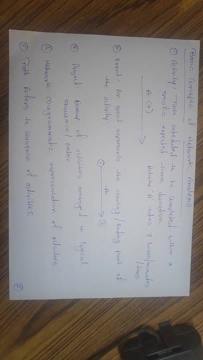 order. That is nothing but a project. Fourth network: a diagrammatic representation of activities is nothing but a network. The path refers to sequence of activities. The path refers to sequence of activities. The path refers to sequence of activities. The path refers activities. A path in a network is nothing but a sequence of activities. 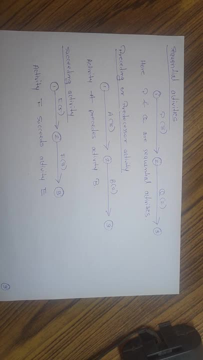 Let's go little deeper. This is some of the practical concepts regarding the network analysis. Now sequential activities. When can we call two activities as sequential activities? Here you can see P, Q. P and Q are sequential activities. P is starting, A will consume. 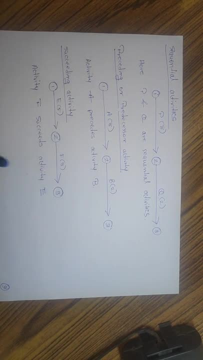 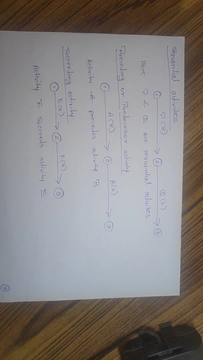 8 units, Q will consume 2 units And P is preceding activity of Q And Q is succeeding activity of P. That's why P and Q are sequential activities In the same way: preceding or predecessor activity- Here preceding activity: Activity A precedes activity B. Very simple Succeeding activity. 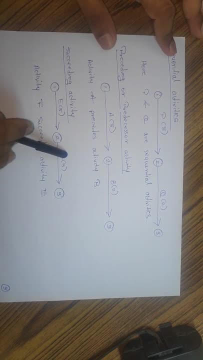 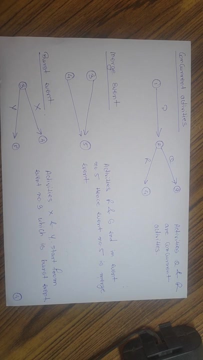 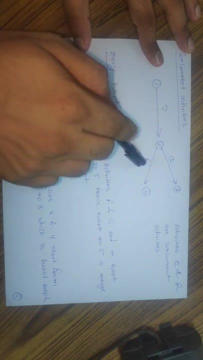 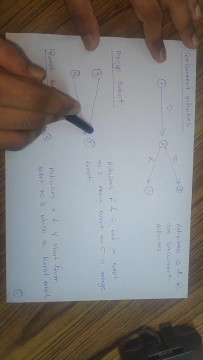 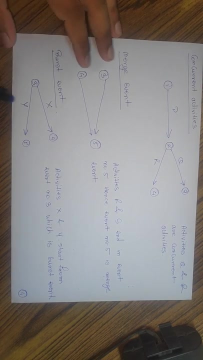 F is succeeding activity E. Two activities are said to be concurrent activities when they start from the same event. Q and R are concurrent activities, In this case. merge event: When two activities merge in particular event, that event is called as merge event. Burst event: When two activities start from one particular event, we call this: 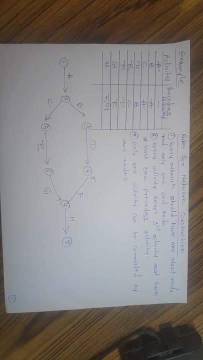 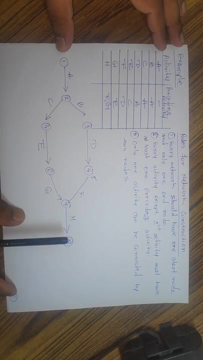 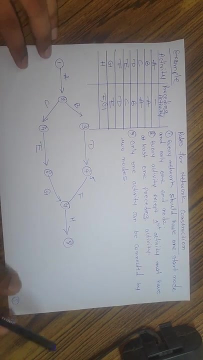 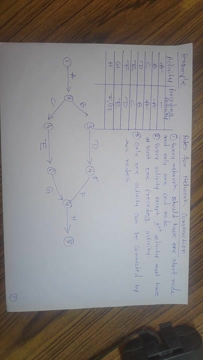 event number 3 as a burst event. Now let's take example. How will you draw the actual network with the help of this given problem? This is a typical example. We will also try to understand the rules of network construction. Let's start. Every network should have one starting node and only one ending node There. 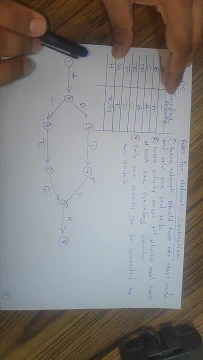 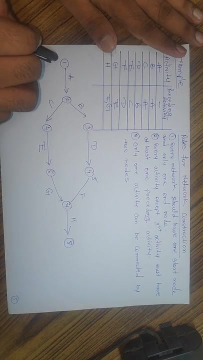 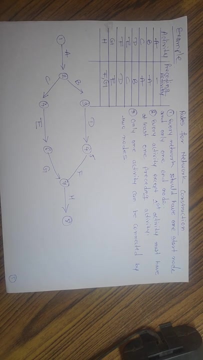 cannot be two starting nodes or two ending nodes. It will start with only one node and will end at one node. One event: one starting event and one ending event, Not more than two events. Every activity, except first activity, must have at least one preceding activity Apart. 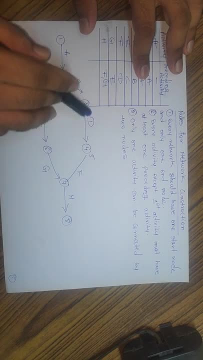 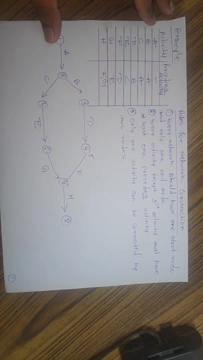 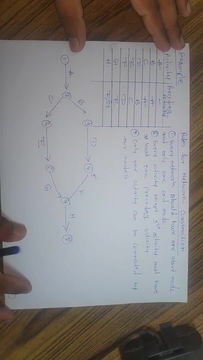 from the first activity, which is A. all activities are having some kind of preceding activity. Only one activity can be connected by two nodes. One activity needs two nodes. We have seen this earlier. So this is the kind of information you will get in the problem Activity. 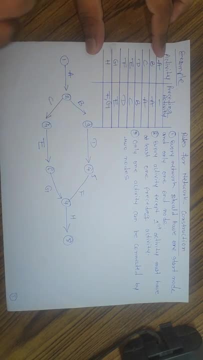 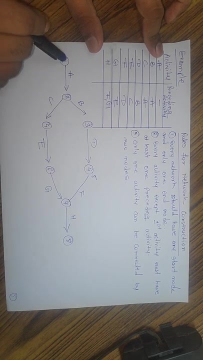 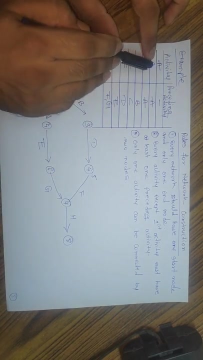 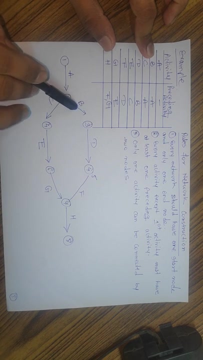 and preceding activity. There is no appropriate activity. that means A is the very first activity. you have to start with 1-2 activity A. Now for activity B, which is the preceding activity A. So activity A becomes preceding activity of B event. but in case of B event it becomes Demonic Representing. Event activity. Who are the second and third activity? Is in the first shadowing event. Who are the third activity? Is in the third shadowing event. Who are the fifth and first activity? Who took the post經� можем? 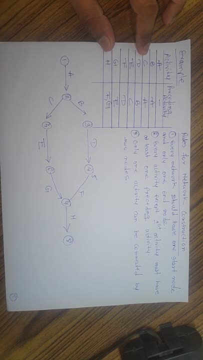 So this event, this activity also has preceding activity as A- That means we will come to know- the event where activity A is ending is nothing but a burst event, Because this event is nothing but a starting point of two another activities, two different activities. 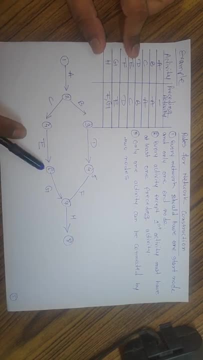 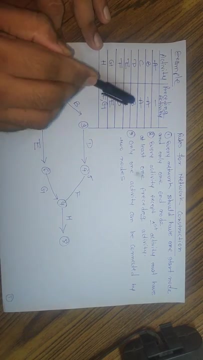 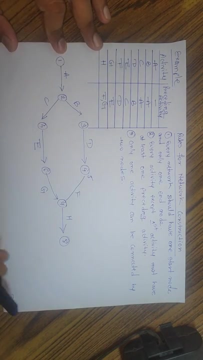 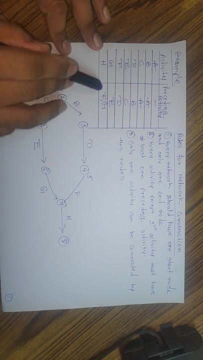 Okay, Then for activity D, activity D: activity D preceding activity is B. This is D preceding activity B. Then activity E preceding activity C. Correct Activity F preceding activity D, F, D, Activity G preceding activity E. For activity H: preceding activities are F and G. From here you can make out: when there are two preceding activities is nothing but a merge event. So two activities are merging in one event. So this is the merge event And H is the last activity. 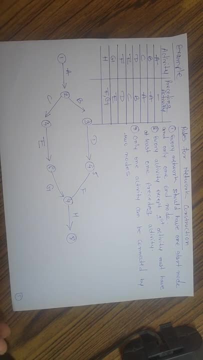 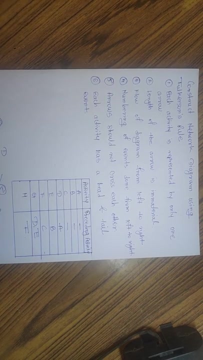 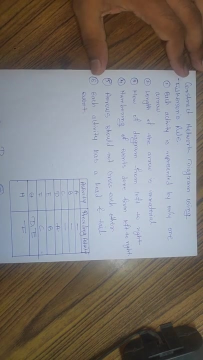 And it will end in event number 8.. Okay, I am taking one more example to clarify some more rules of the network construction. This is called as Fulkerson's rule. First rule is very simple. Each activity is represented by 1.. 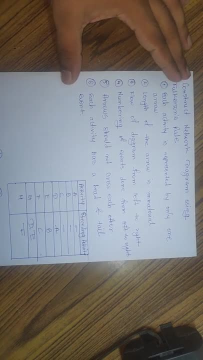 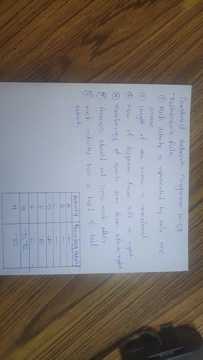 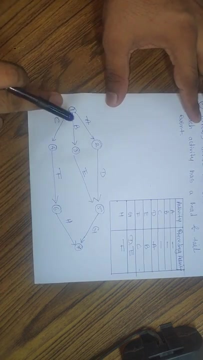 One arrow, Only one arrow. Length of the arrow is immaterial. Whether you draw a long arrow or a short arrow, it doesn't matter, because the length of the arrow is immaterial. Flow of the diagram from left to right, From left to right. 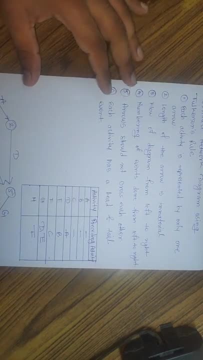 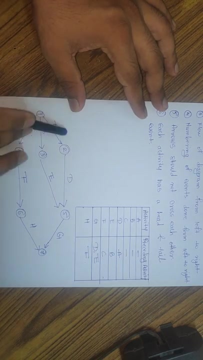 This is the flow of diagram. Network diagram from left to right. Numbering of events done from left to right. Numbering of events will be done from left to right. Arrows should not cross each other. No arrow should cross each other. 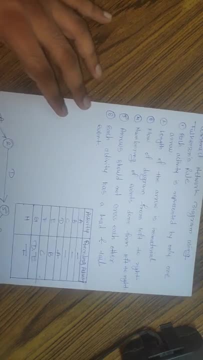 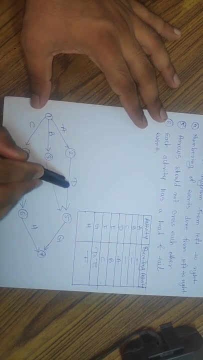 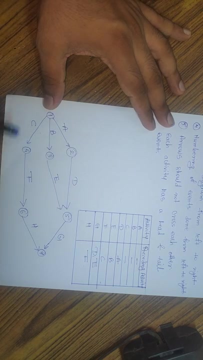 Crossing of arrows is not allowed. No arrow is crossing each other. Each activity has a head and tail event. Each activity, any activity, let's say E activity, has 1 tail event 3 and 1 head event 5.. Okay. 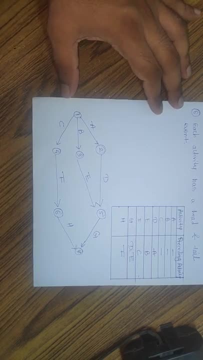 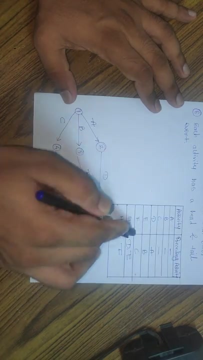 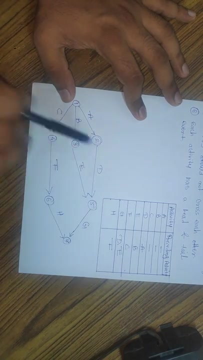 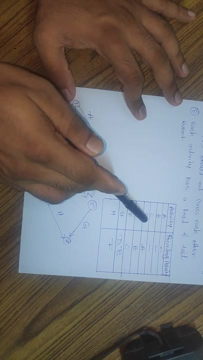 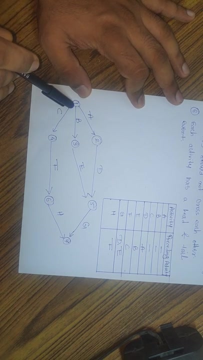 Okay, Now let's try to understand how this network diagram is drawn. this is the kind of data or information you will have with you: activity and preceding activity. just look at the activities a, b, c. okay, and there is no preceding activity for activity a b c. that means there is a starting event is: 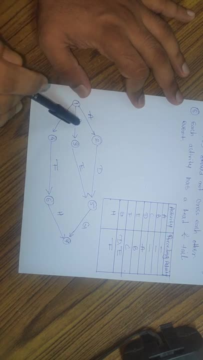 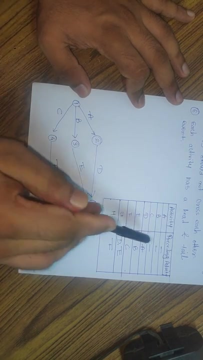 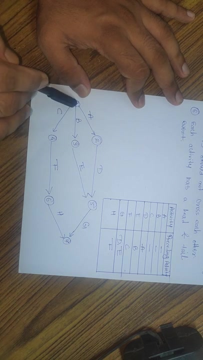 burst event for these three activities, BC. these three activities are starting from only one event, number one: A, B and C. okay for activity. the preceding activity is a. this is the preceding activities was keep in mind left-to-right. you have to number the events from left to right. the flow of diagram is from: